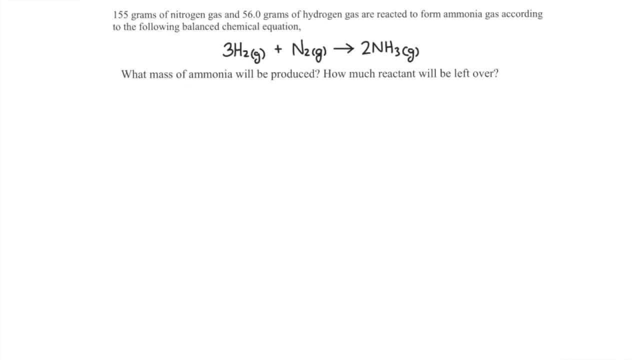 used in a lab and in a chemical factory. so let's look at a more complex problem. This rule says 155 grams of nitrogen gas is required gas and 56 grams of hydrogen gas are reactant to form ammonia gas. What mass of ammonia gas? 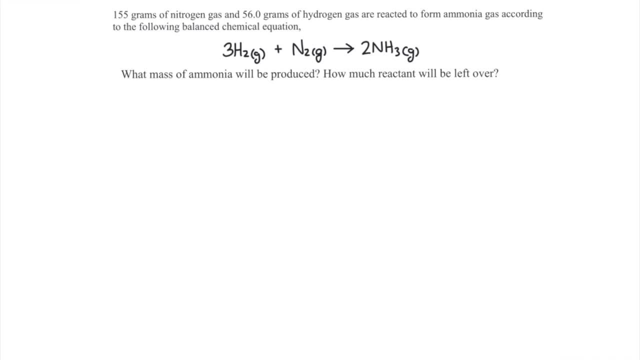 will be produced and how much reactants will be left over. This problem involves a limiting reactant, because the quantities of two reactants are given. There are two ways to solve a limiting reactant problem like this. We could first compare the two reactants to each other and determine. 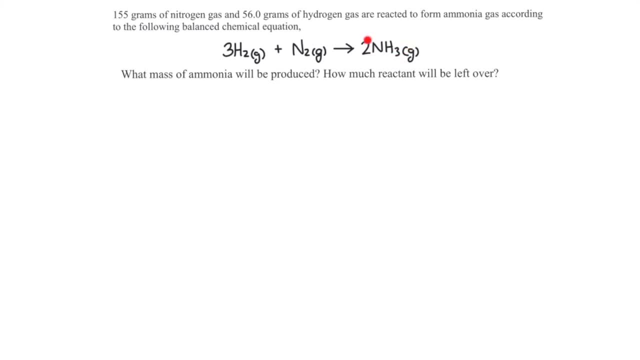 which one runs out first, and then use that to figure out the amount of product that could be made. Or we could determine the amount of product that could be formed by completely consuming each reactant, like calculating two separate problems, and then we could compare the amount of product. 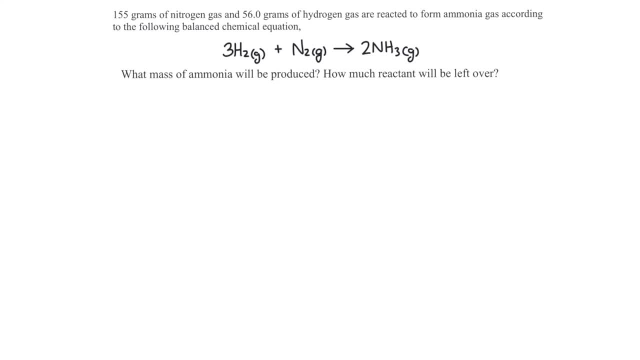 formed by completely consuming the first reactant to the amount of product formed when completely consuming the second reactant. Whichever gives the smaller amount of product, that will be the limiting reactant. I'm going to solve this problem using that second method. If 155 grams of nitrogen is consumed? how much ammonia gas does the reactant produce? How much carbon dioxidesubmits the К2 element of CO2 into it? Let's try the first method. If 155 grams of nitrogen is consumed, how much for the Randor hydrogen being dissolved? so thisаются to 50 grams of ammonia gas? What amount ofимся to 155 grams? 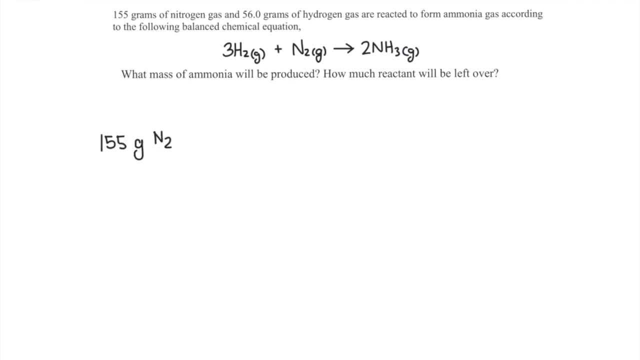 would be produced. First we'll convert the mass of nitrogen gas to moles and then we'll compare that to ammonia by multiplying by the mole ratio. To convert 155 grams to moles, we will divide by the molar mass of nitrogen gas. Nitrogen gas is N2.. There's two nitrogen atoms and each nitrogen. 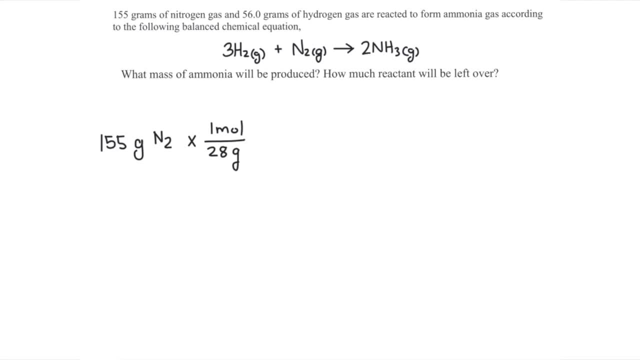 atom has a molar mass of 14.. So the molar mass of nitrogen gas is 28 and the mole ratio that compares ammonia gas to nitrogen gas is 2 to 1.. There will be two times the amount of ammonia compared to the amount of nitrogen gas, based on the chemical equation 155, divided by 28 times. 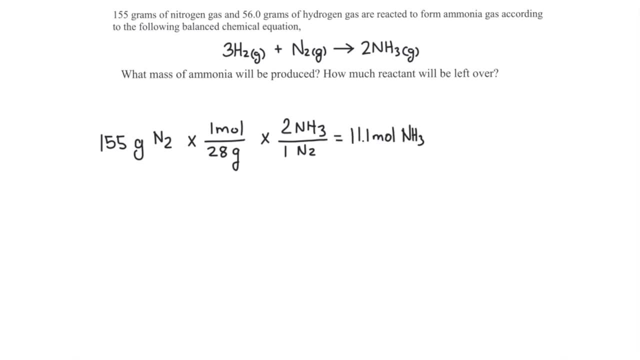 2 over 1 gives 11.1 moles of ammonia gas. Since the question is asking for our answer to be in mass, we're going to convert that 11.1 moles of ammonia gas into grams by multiplying by the molar mass of ammonia. The molar mass of ammonia is N2.. We're going to convert that 11.1 moles of 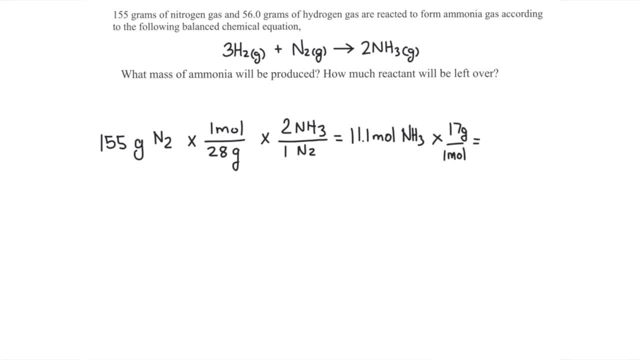 ammonia gas would be 17.. So 11.1 moles times 17 gives us 188 grams. Now we're going to do the same type of calculation, but we're going to use the 56 grams of hydrogen gas, 56 grams divided by. 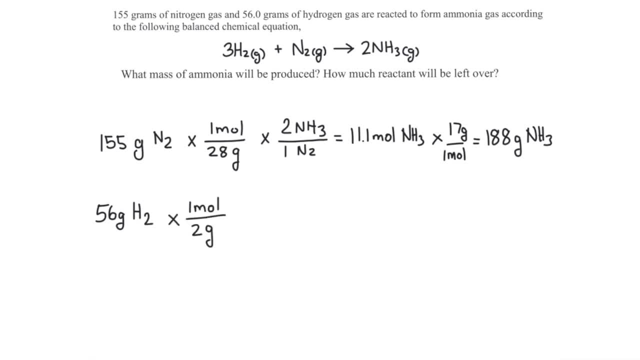 the molar mass of H2, which is 2 grams per mole, times the mole ratio, which is 2 over 3, gives us an answer of 18.7 moles of ammonia. We're going to multiply this by the molar mass of ammonia. 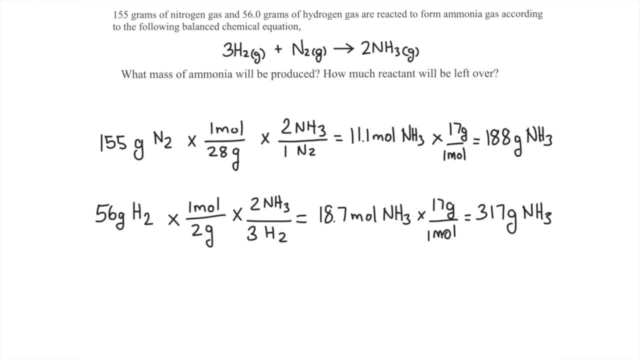 to give us N2.. We're going to multiply this by the molar mass of ammonia to give us N2.. We're going to multiply this by the molar mass of ammonia to give us 317 grams. Now we're going to compare these two answers, Since 155 grams of nitrogen gave the smaller amount that means. 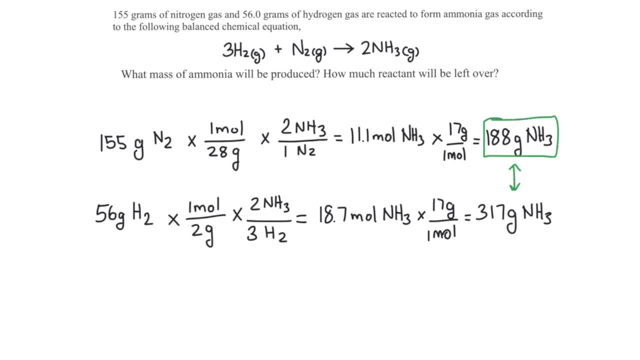 nitrogen is the limiting reactant. Nitrogen runs out first in this chemical reaction. So we can answer the first part of this question by stating that 188 grams of ammonia could be produced when 155 grams of nitrogen reacts with 56 grams of hydrogen gas. The second part of the question, 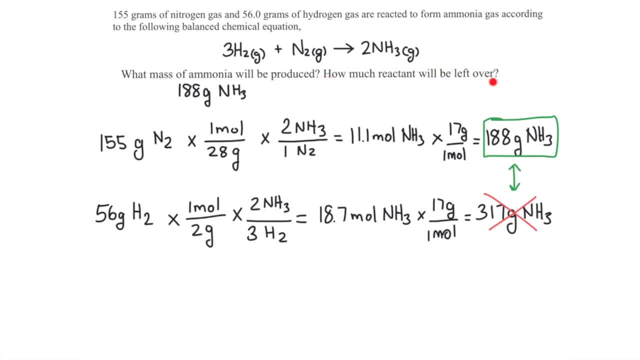 asks us how much reactant will be left over. We're going to multiply this by the molar mass of ammonia to give us N2.. Well, nitrogen is used up completely, and so there will be some hydrogen left over. How much hydrogen is left over depends on how much was used in the reaction We need to determine. 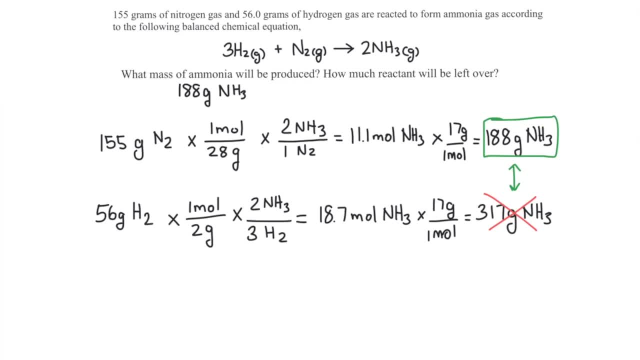 the amount of hydrogen that was used by comparing the amount of nitrogen that was used. All 155 grams of nitrogen was used up. I'm going to convert that to moles and then compare it to hydrogen by multiplying by the mole ratio 3 over 1.. I'll convert that to grams of hydrogen by multiplying. 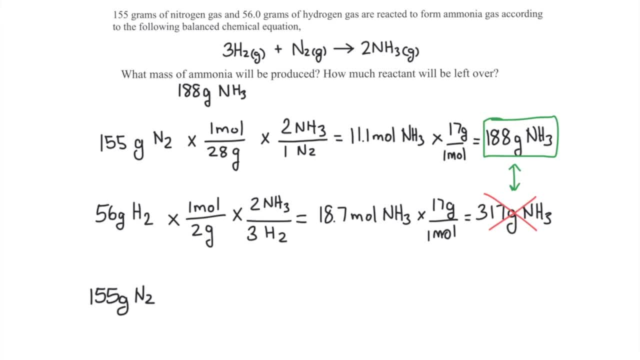 by the molar mass of hydrogen, and I'll determine exactly how much hydrogen was used. 155 grams divided by the molar mass of nitrogen times the mole ratio of 3 over 1 times the molar mass of hydrogen, which is 2 grams per mole, gives us 33.2 grams. 33.2 grams of hydrogen gas. 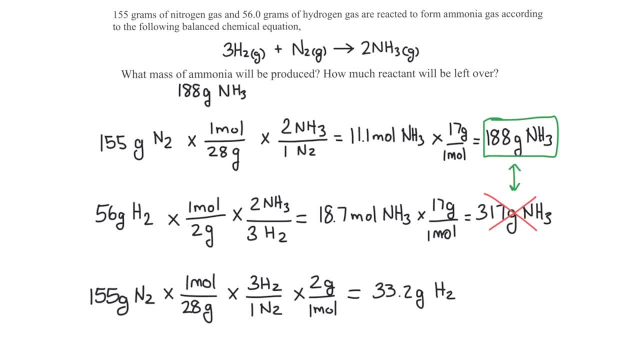 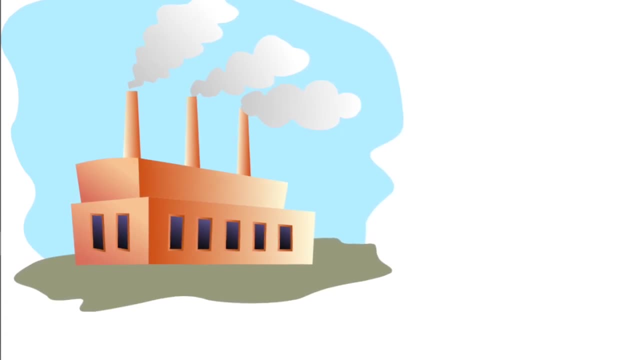 was used up and we started with 56 grams. So the amount left over will be 56 grams subtract 33.2 grams, which gives 22.8 grams of hydrogen gas left over. There are large factories that produce ammonia using the equation we saw in the previous example. These factories want to make money and produce as much.